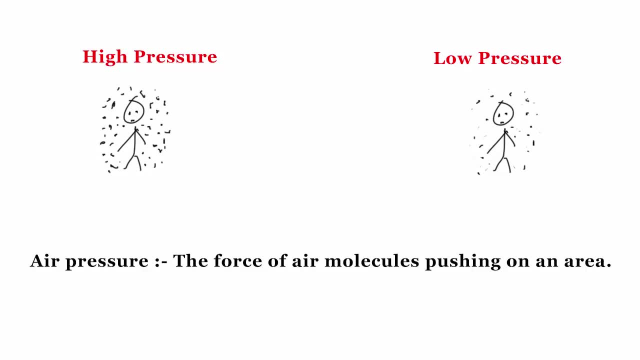 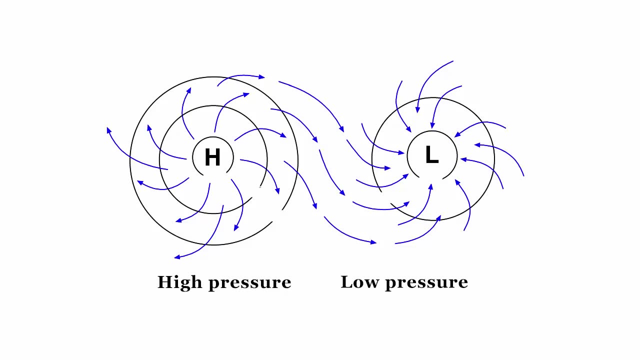 wind system. By pressure we mean high and low pressure system. Always remember, air moves from high pressure to low pressure area, The best way to understand this. I have given this illustration before, so I'm going to use it again. Switch on the AC in your room and leave the door open. 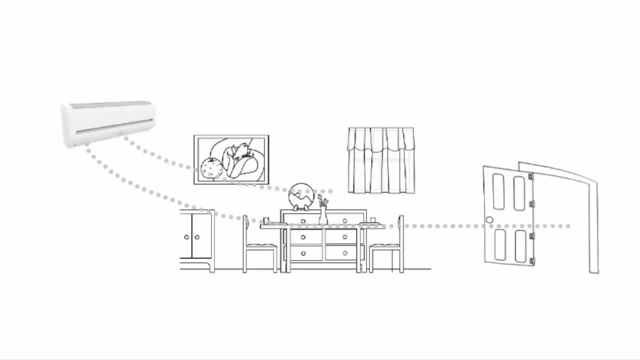 You will feel the cool air going out of the room, and this is because the environment outside your room is warm and it's attracting the cool air molecules towards it. Hence, by this example, you can also understand this. Landmass gets heated faster than water bodies, And due to that, 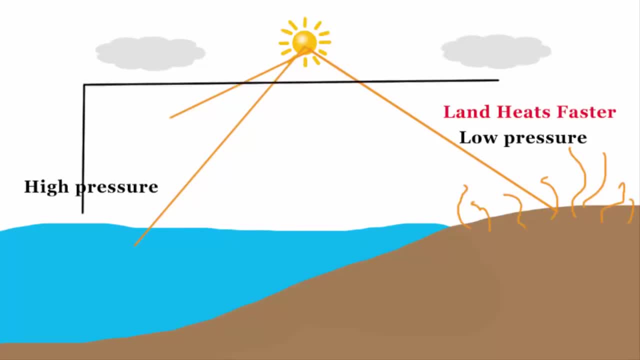 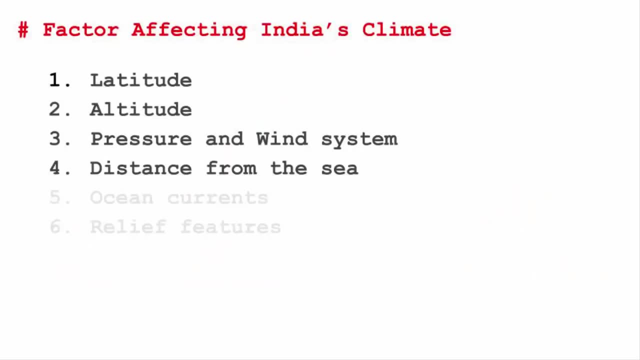 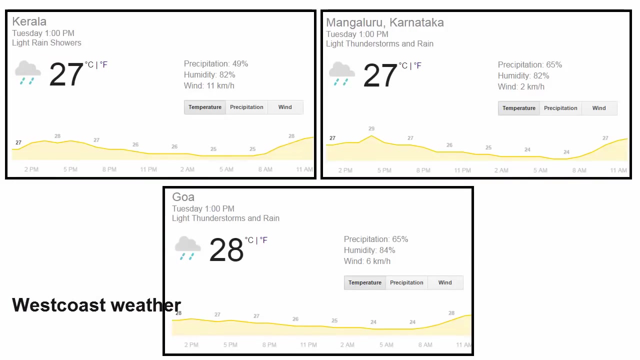 a low pressure zone is created at the land surface which attracts cool air molecules from the sea or ocean, causing rainfall and changes in the temperature. The fourth factor is distance from the sea. Now, if you are residing at coastal areas, you will notice there is hardly any change in the weather condition. I mean you will be constantly. 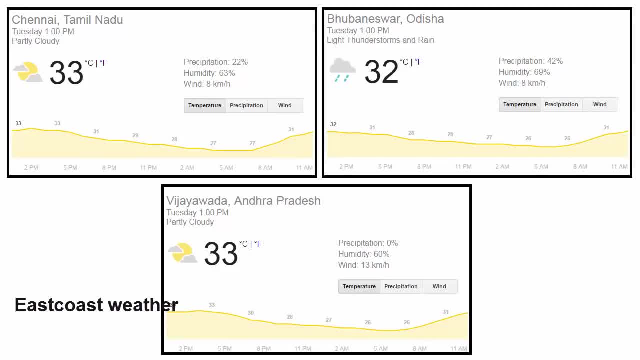 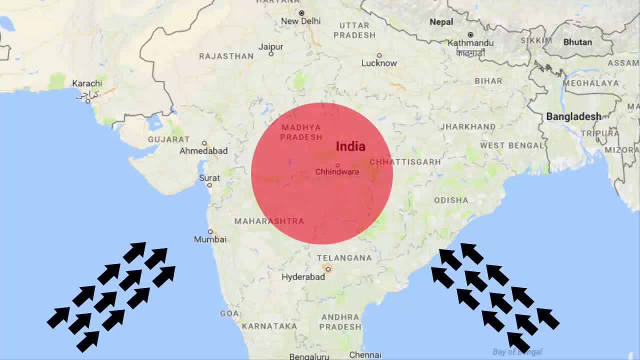 facing the wind from the sea, so there isn't going to be much differences in the weather condition. But as you move away from the coastal areas towards central part of the landmass, you will start to witness extreme weather changes like very hot during summer and very 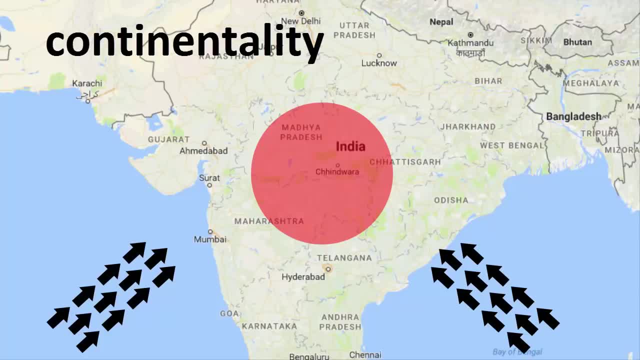 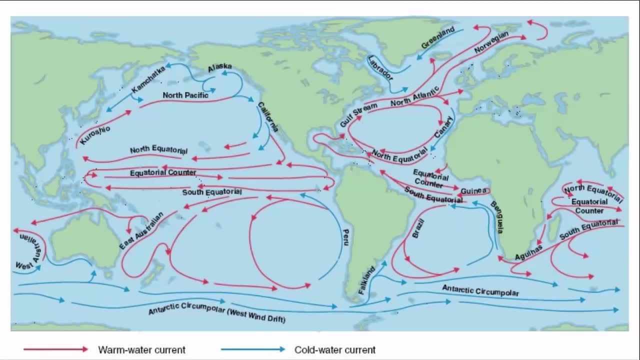 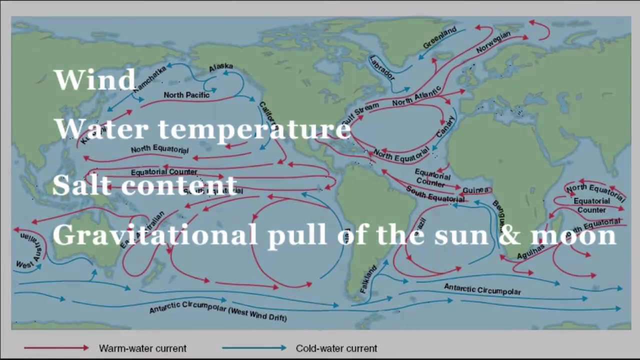 cold during winters. This condition is known as continentality. The fifth factor is ocean currents. It is a continuous movement of ocean water from one place to another. Ocean currents are created by wind, water temperature, salt content and the gravitational pull of sun and the moon. Generally, there is two types of ocean currents. 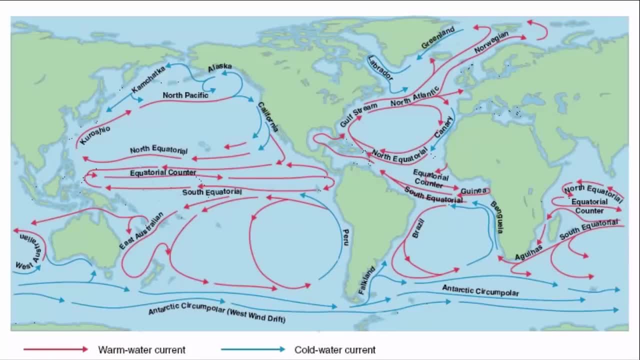 cold and warm currents. You can see them in this picture: The red arrow indicates warm currents and the blue one are cold currents. If you notice, most of the warm currents are near the equatorial region. That's where the sun rays falls directly and are found in abundance. 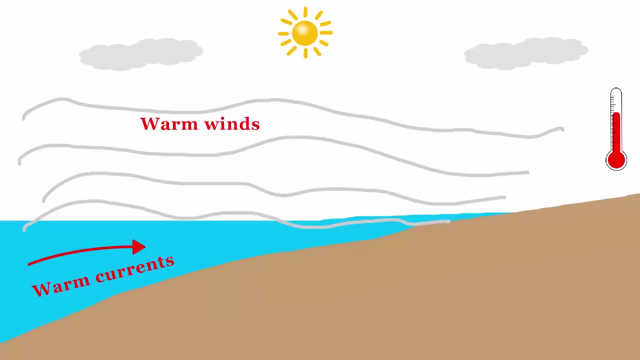 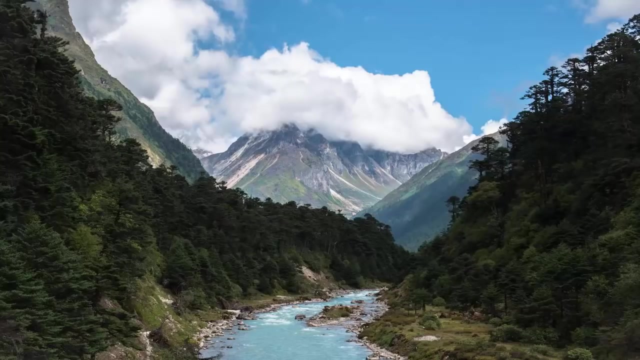 The theory is these warm and cold current influences the local winds of the nearby landmass and causes change in the climatic condition. For example, with warm currents the landmass face warm and humid climate And the last factor is relief. features In geography. the meaning of. 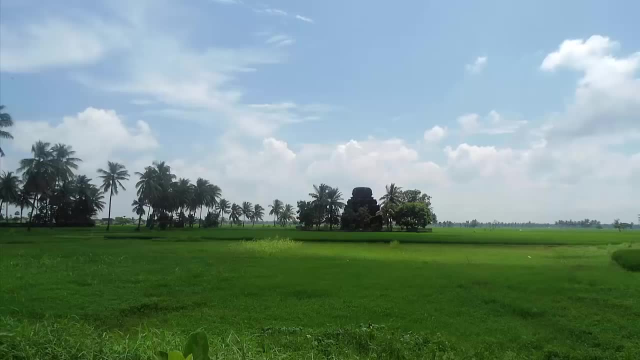 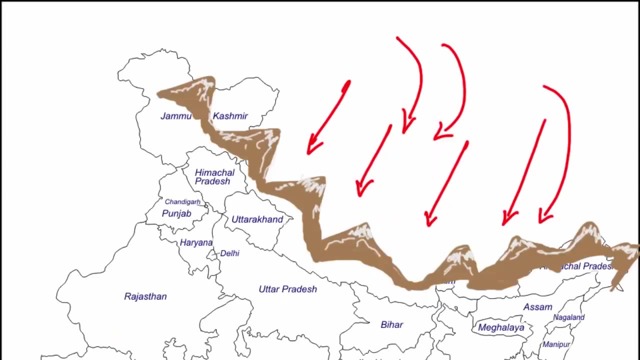 relief is typical high and low lying areas like mountains, plateau plains, deserts, etc. High mountains act as barriers for cold or hot winds, just like we have the Himalayas that protect us in the Arctic, And it is also due to these mountains precipitation takes place. One such